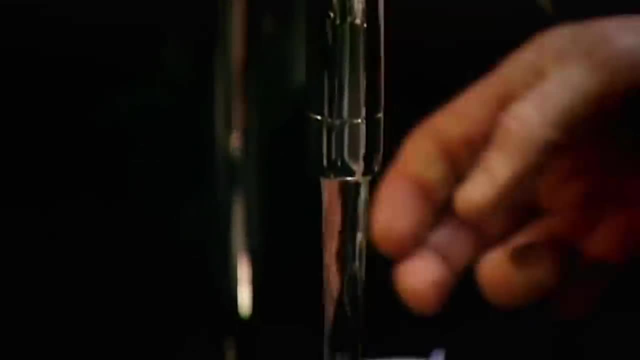 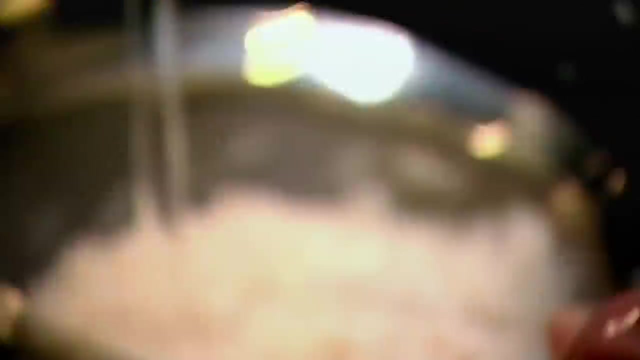 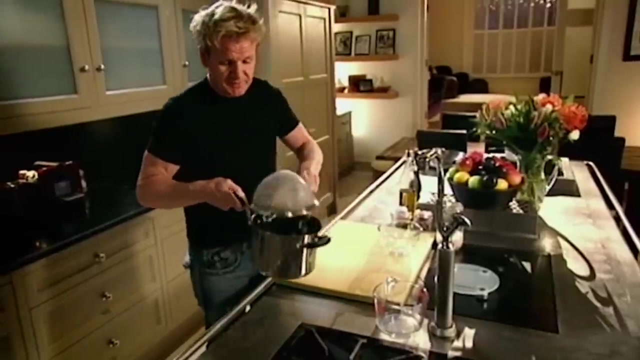 do now is just rinse off the dust and the starch. Cold water always- And just rinse the rice. That stops the rice from becoming clumpy in the pan and allows it to become really nice, light and fluffy once it's cooked. Rice into the pan. Now to make a plain fluffy rice- exciting, we're going to. 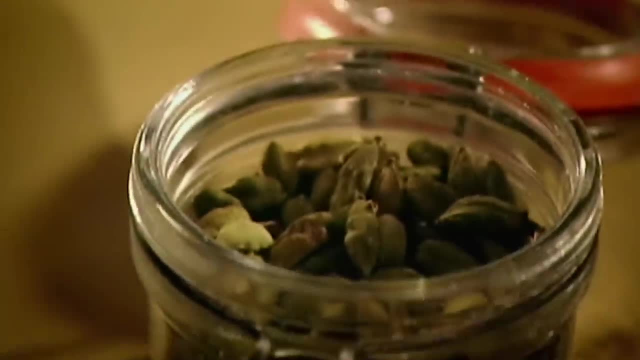 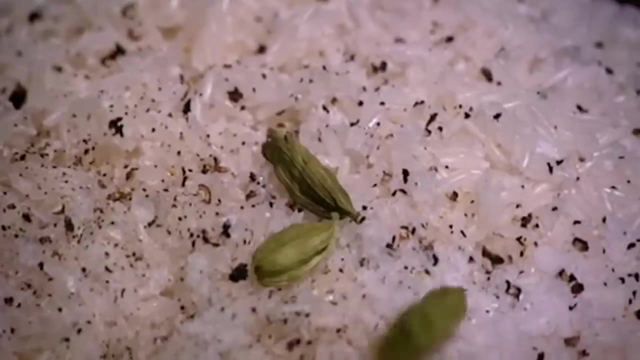 infuse it Three cardamom pods And just get the pods and just pierce them so it allows all that flavor to come out. Cardamom pods And then star anise. Now these are beautiful Whole star anise. 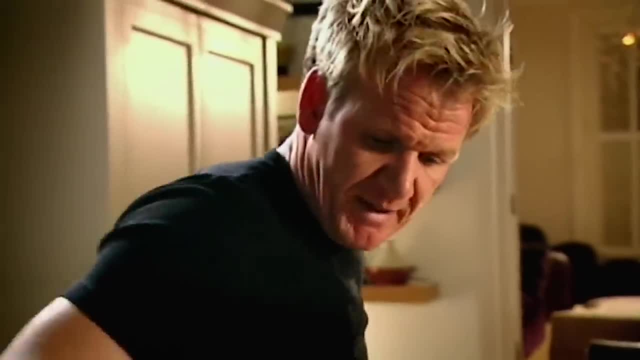 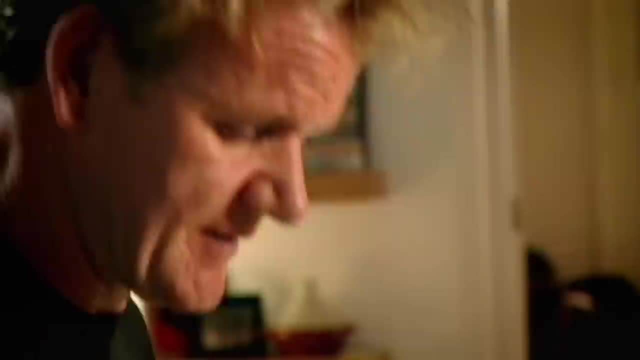 It makes it really nice and fragrant. Salt and pepper. A lot easier to season the rice now than it is once it's cooked. You start to break it up when you season it once it's cooked. Now, basically, one part rice to one and a half part water- 600 mils. Always start off in cold water. 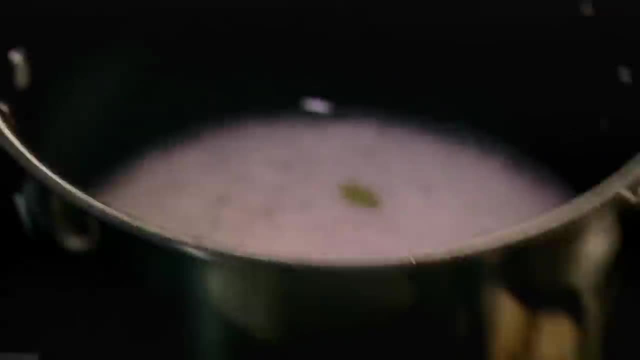 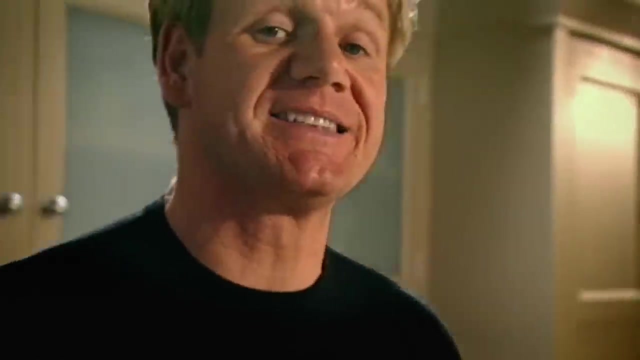 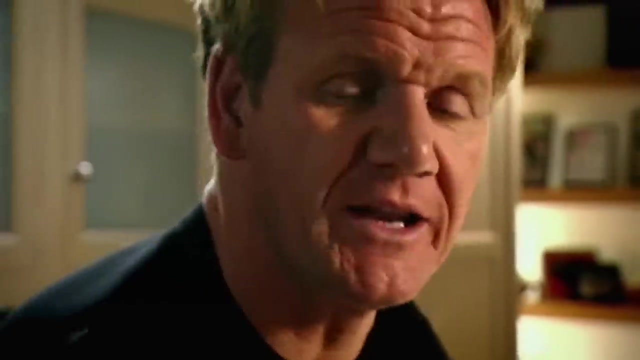 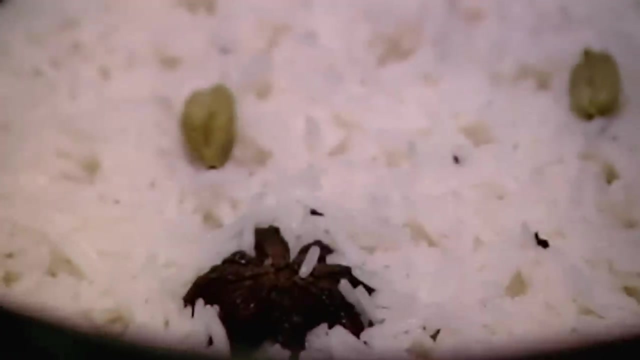 Cold water in Onto the gas Lid on, Bring it up to the ball as quick as possible and turn it down and let it simmer for eight to ten minutes. And that's the secret behind cooking great rice. Allow it to steam as it's cooking. Do not lift that lid up, Lid off. Mmm, It smells aromatic. 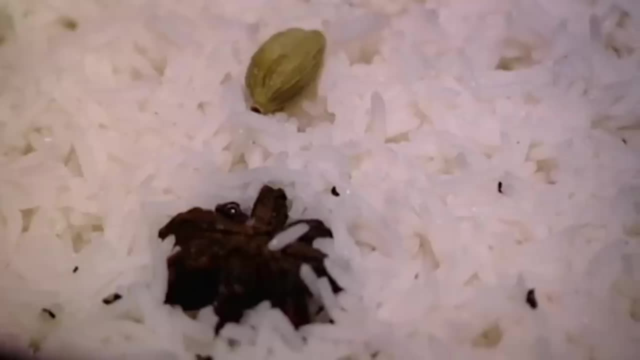 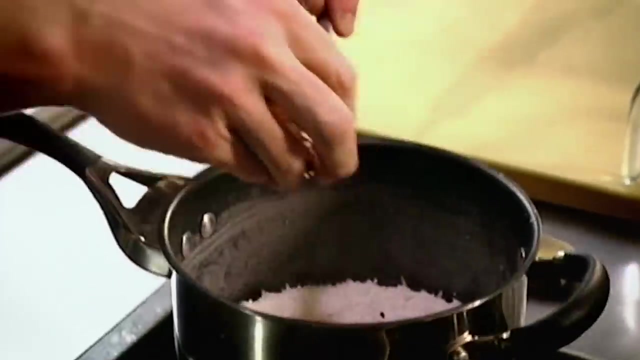 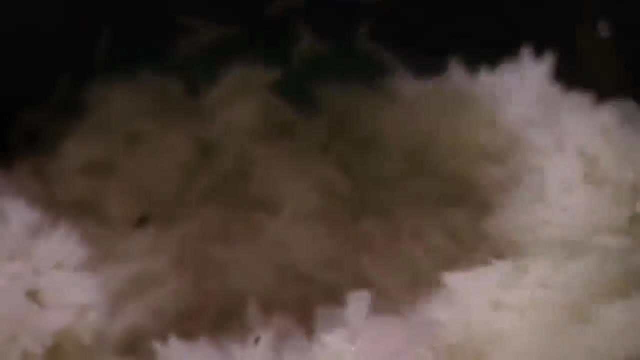 Basically all the water's absorbed. The rice has doubled in size and it's nice and light and fluffy. Take the star anise out The cardamom pods- They all should have risen to the top- Pods out. Take your fork, Fluff it through. Basically, it just sort of starts to open everything back up. 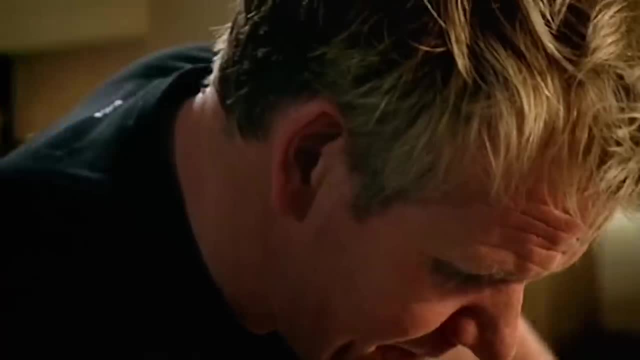 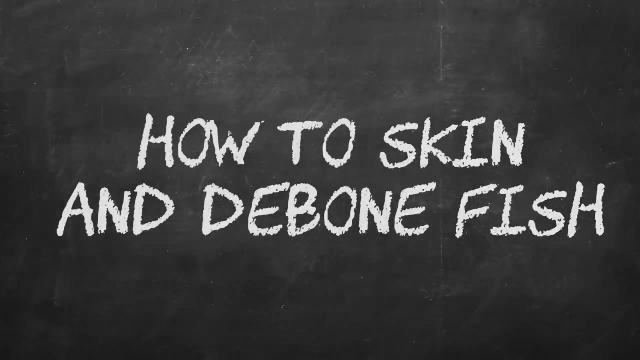 Once you've forked it through, it becomes really nice and light and fluffy, And there That is perfectly cooked rice. This is basically a filleted side of salmon. This is basically a filleted side of salmon. This is basically a feeded side of salmon. 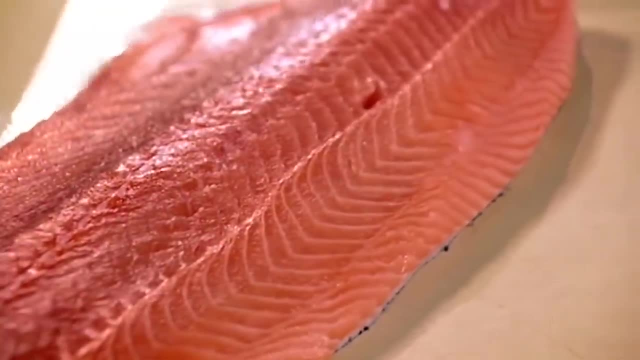 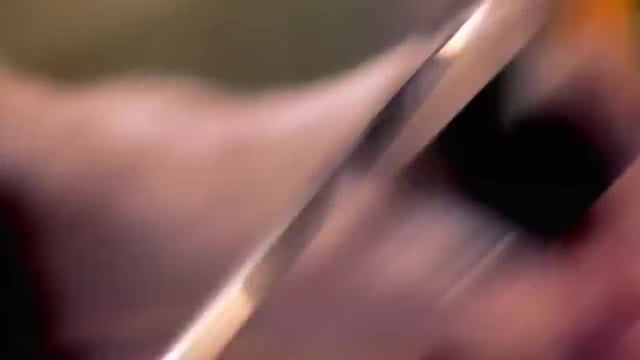 This is basically a filleted side of salmon. This is basically a filleted side of salmon. It's been taken off the bone and now skin off. Pick up your knife- a really nice, broad, flexible filleting knife, Little sharpen. lift up the base of the tail. 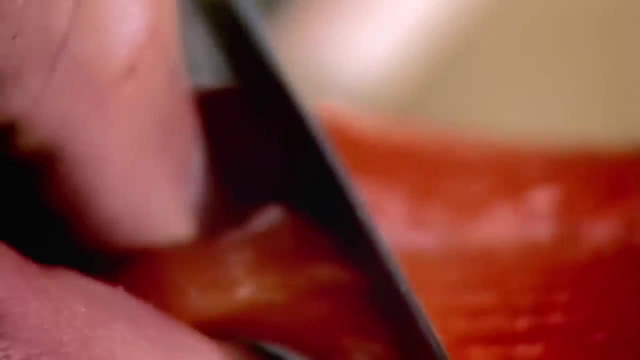 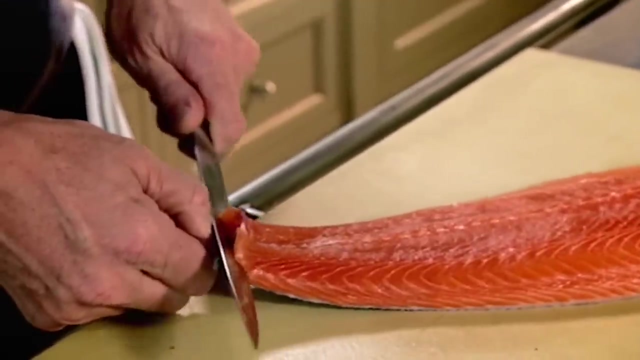 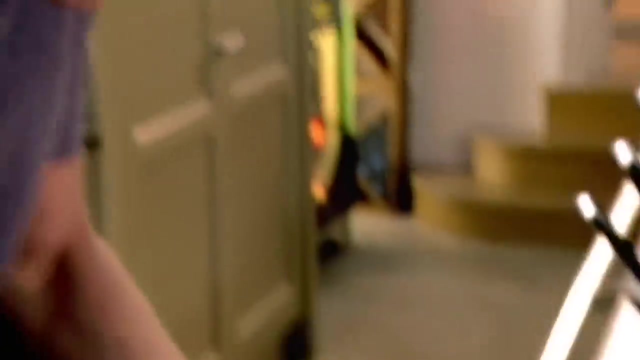 and then just nick a little bit at the end. there Twist the knife almost as if it's horizontally underneath the salmon. Pull the skin and you slice the salmon underneath and let the knife do the work. Now get your skin, flip it back over. 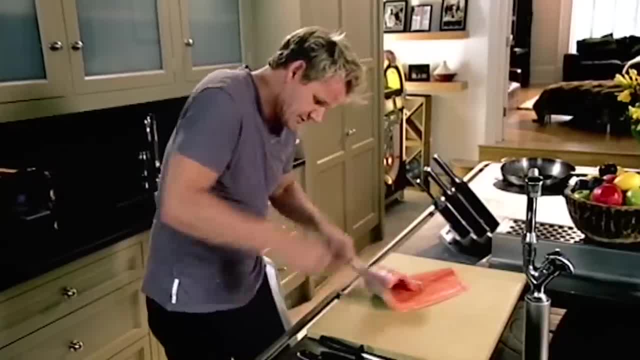 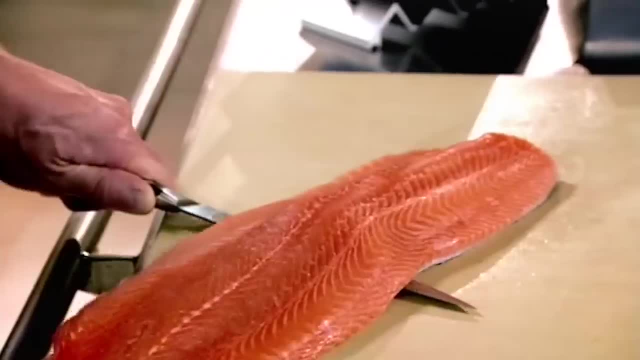 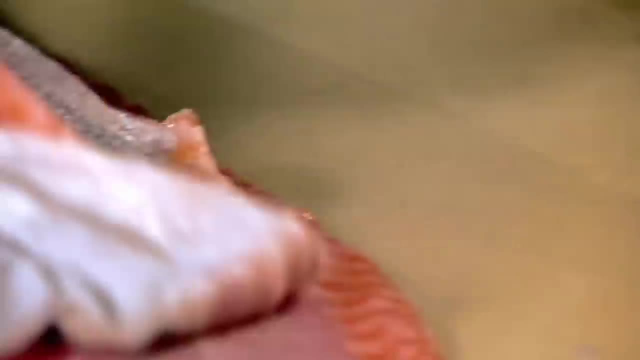 and check you're not leaving too much salmon on top of the skin. Pull it back and nice and slowly get the skin, wrap it around your fingers, pull the salmon towards you and then, just all the way through, Lay that down: one nicely skinned salmon. 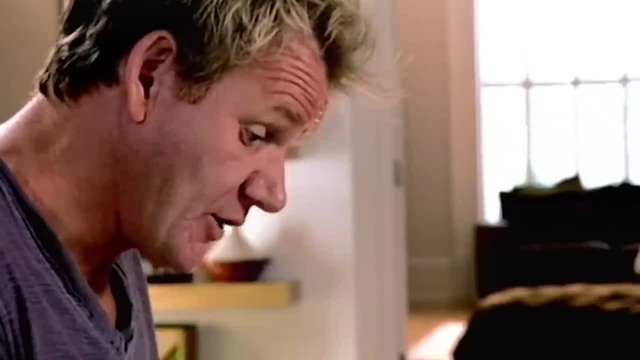 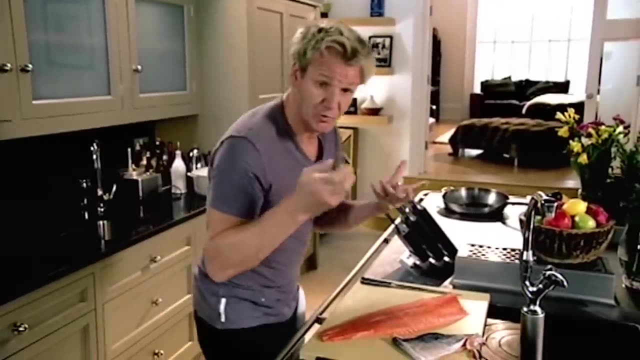 just like a perfect snakeskin. Get your knife Now, just run the knife down and then with a pair of tweezers- these are fish tweezers, but you can use normal tweezers- look for the head up and pull. 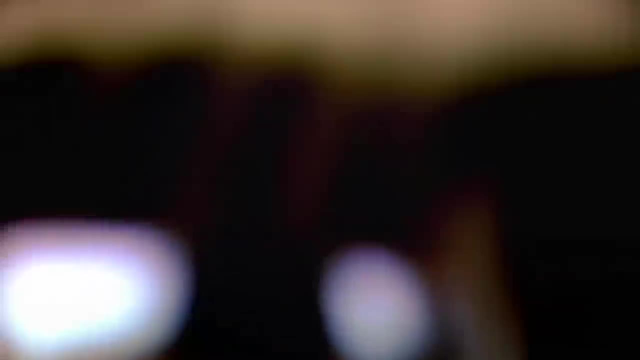 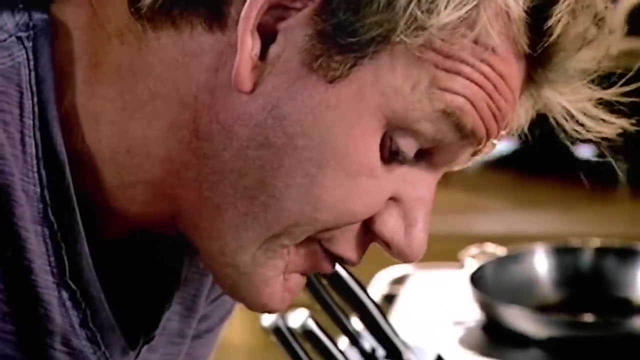 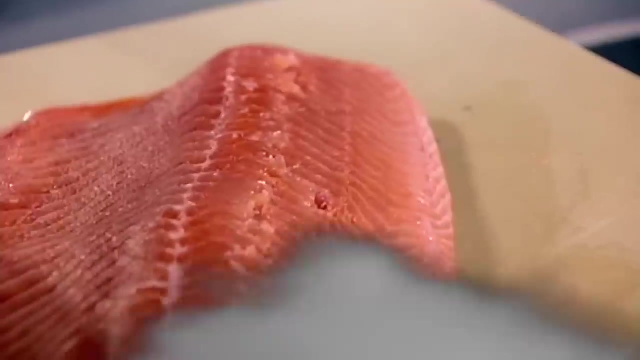 And with the skin being removed from underneath the salmon, the pin bones come out a lot easier. The pin bones only go to just basically halfway along the fillet. One nice fillet of salmon, beautiful. It's far harder working in the kitchen with a blunt knife. 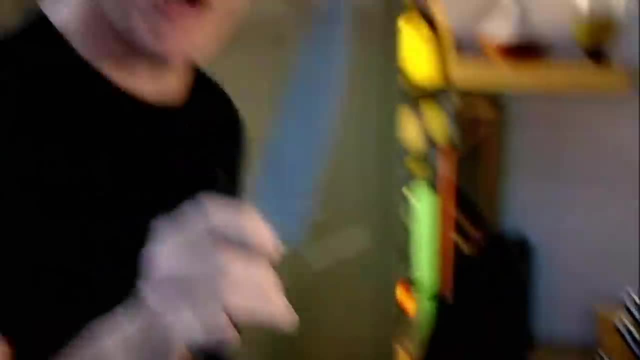 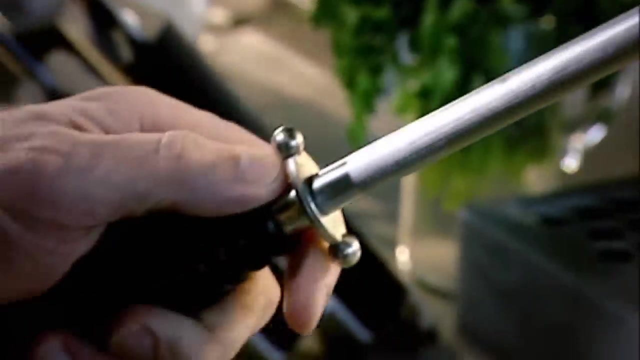 than it is with a sharp knife. The secret behind keeping a sharp knife: sharpen it before and every time you use it First, grip the steel. Feel really comfortable about holding the steel. Imagine you're holding a tennis racket or you're playing squash. 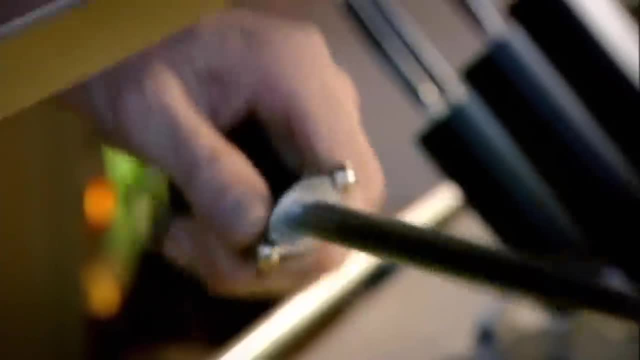 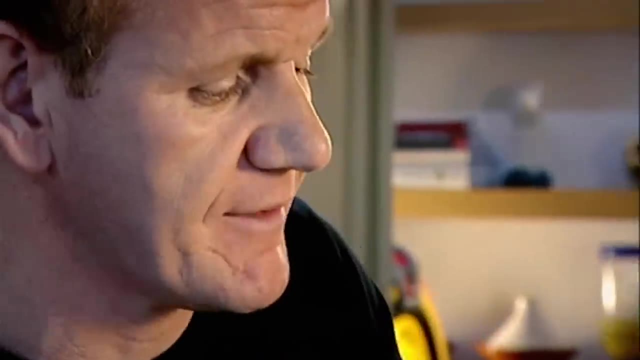 You've got to be really comfortable with it Now. 45 degrees, confident grip, confident grip with the knife. This is the butt of the steel, Really important to keep your fingers behind that. You never grip a steel with your fingers over that because, oh, oh. 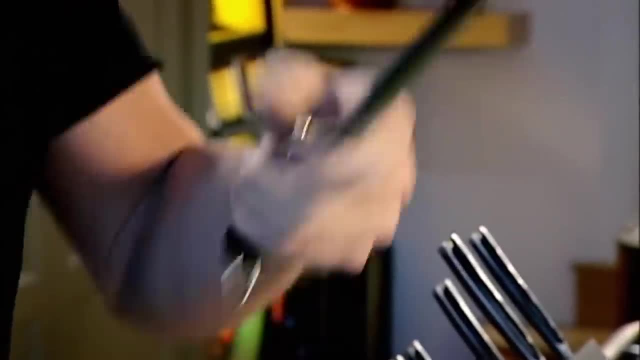 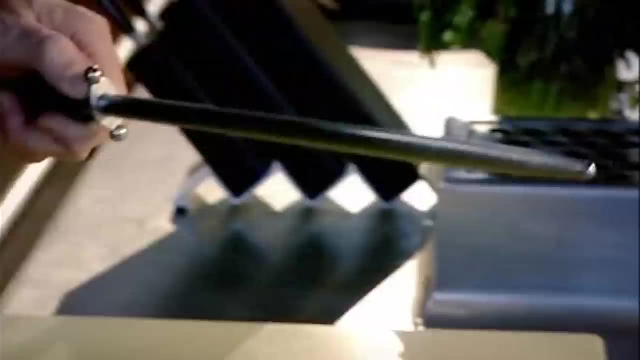 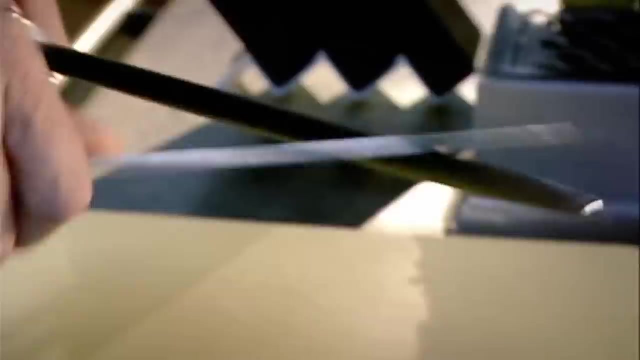 The knife comes back in. You've just lost a finger. Always grip behind Nice long strokes. so we get the hole of the blade over the steel Stroke And we start from the bottom to the top. So there across, there across. 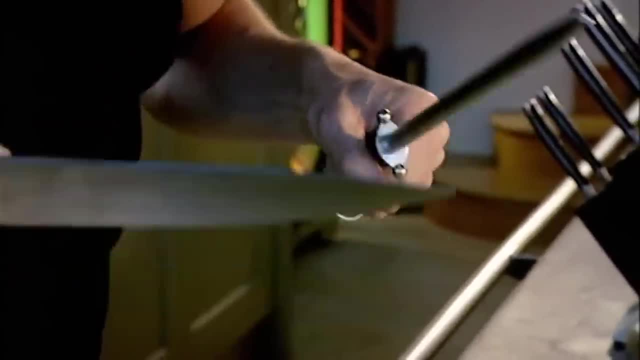 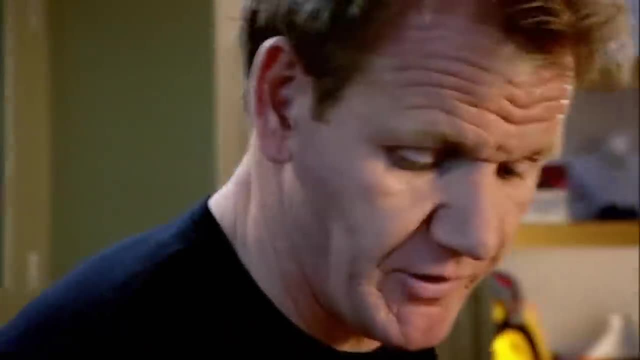 Slow strokes over the top of the steel And then come back underneath, Then back underneath. It is so dangerous working in the kitchen with a blunt knife- Enjoy Like blown mean knife. It can cause so much damage. Working with a sharp knife is ten times quicker, more.